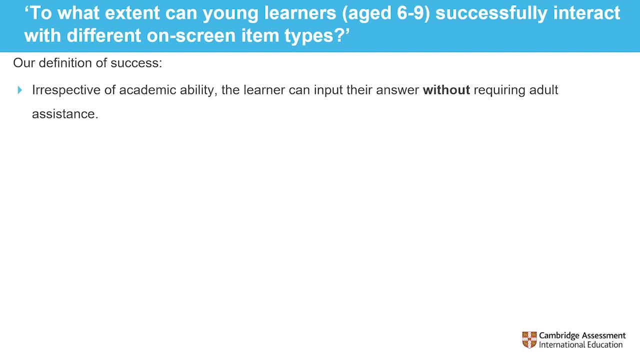 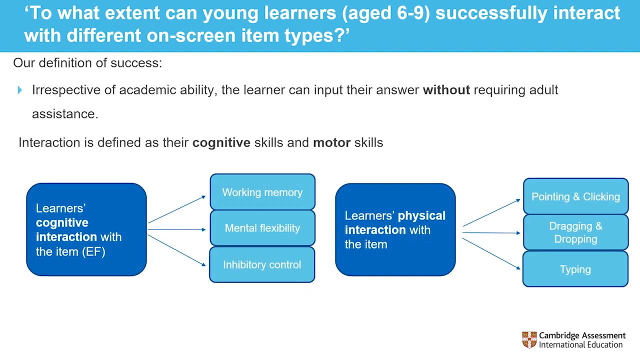 And through this, our definition of success was that, irrespective of academic ability, a learner can input their answer within the on-screen assessment Without requiring any adult assistance or input. With regards to defining interaction, we are looking at cognitive skills and motor or physical skills of the learner. learners cognitive interaction. 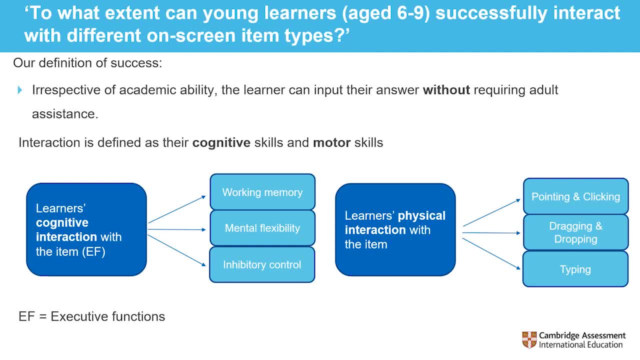 By this we mean that executive funding pockets of cash, Make sure and translate, If necessary, executive functions, including their working memory, mental flexibility and inhibitory control. What cognitive skills do learners of this age have, and how do these impact their interaction? 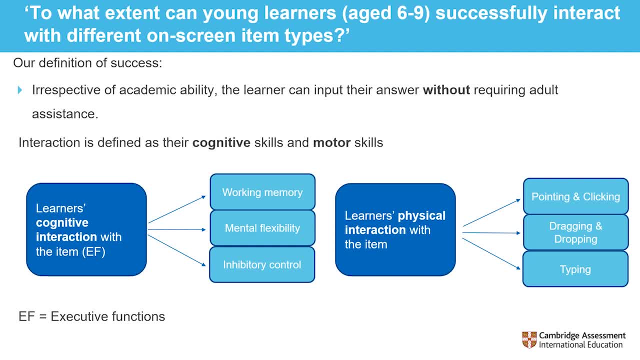 with on-screen items And the expectations about how to input their answer. We might ask the same question for paper-based assessments, but for on-screen the layout is different, the cognitive load might change and the command words do not fit the expected action With respect to motor. 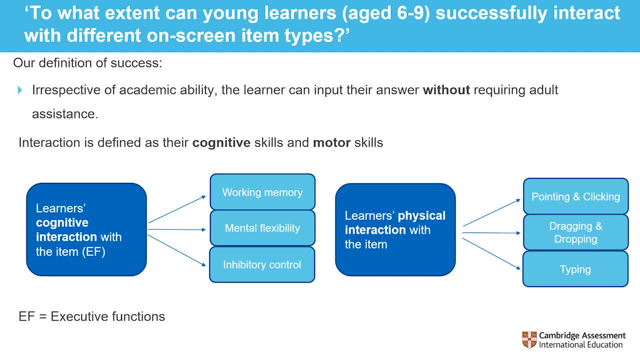 skills. asking what young learners can physically do. how much can they type compared to write? how accurate can they drag and drop? can they easily point and click on screen? If a child requires assistance with a particular item type in order to input their answer, whether this be. 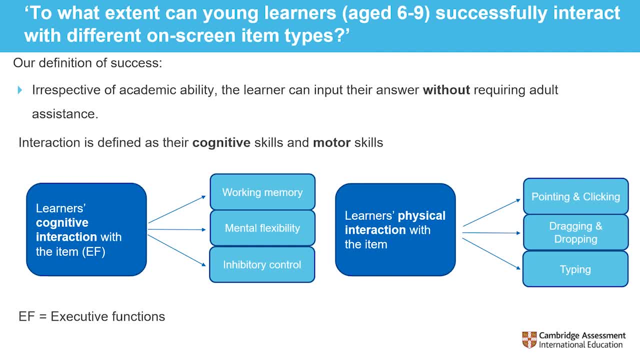 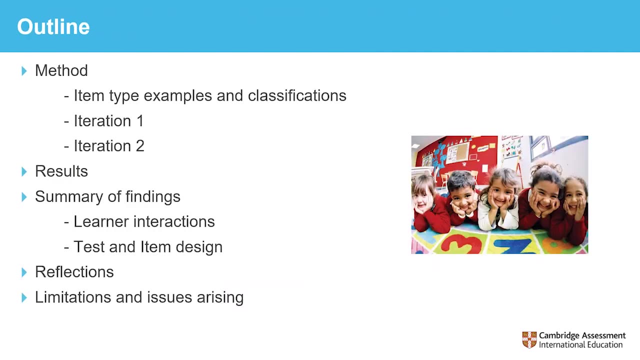 due to motor or cognitive skills, then this is a threat to the validity of the assessment. There should be no barriers to learners being able to demonstrate their knowledge, and it's our responsibility as test developers. So during this presentation, I will briefly cover the method that was used, defining the item types. 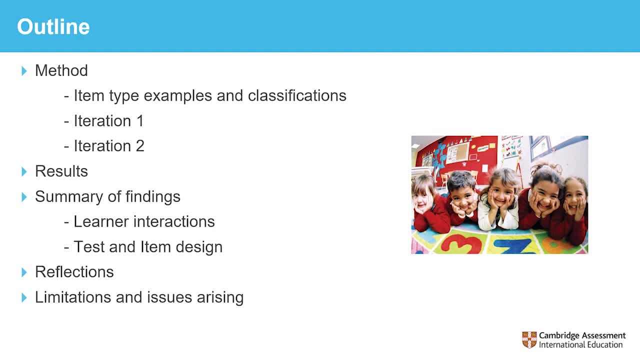 used and how they were classified. Secondly, the two phases of iterations of the trialling. This will be followed by a brief overview of the results that came out, covering some of the statistical methodology used. I'll report on the high-level findings across the 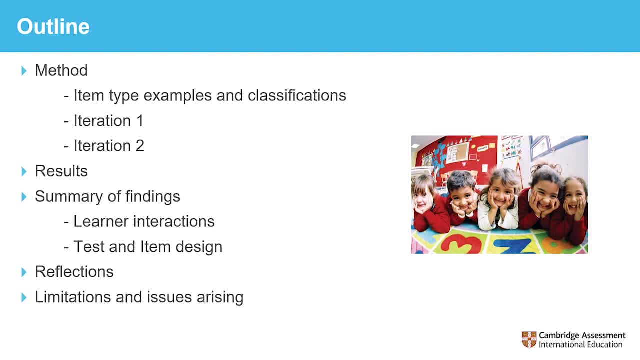 two areas: aspects relating to learner interactions and the item types, and then findings around the design of the on-screen tests and items within them for younger learners. Finally, I will conclude with a brief reflection slide focusing on digital literacy and follow-up, with some limitation and 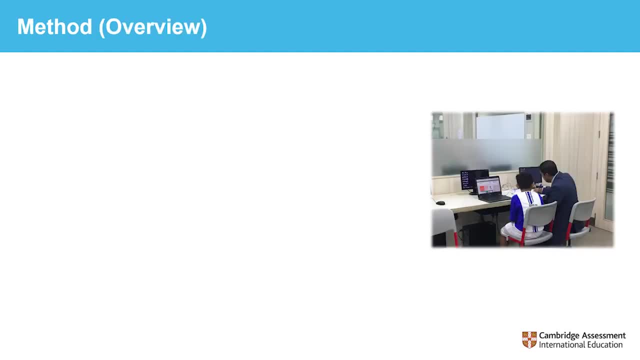 issues arising. With regards to the method, here is an overview of what we did. The first part was to carry out extensive desktop research. The desktop research was split into four parts: sorting academic research, looking at previous internal work and looking at the results. The first part was to carry out extensive desktop research. The desktop research was split into four parts: sorting academic research, looking at previous internal work and looking at the results. The second part was to carry out extensive desktop research. The first part was to carry out extensive desktop research. 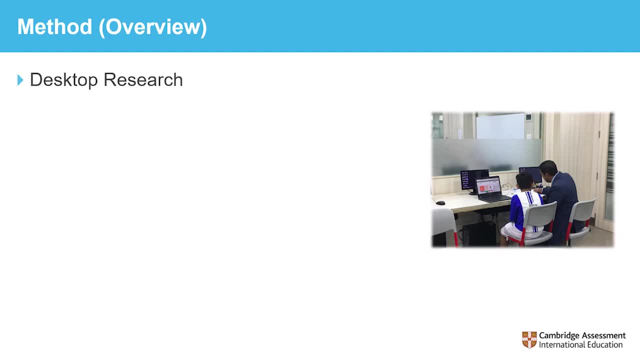 Looking carefully at paper-based or on-screen item type translation work and, finally, looking to the assessment delivery platform, which the one we used was called Inspira. Secondly, as we knew the question we were to answer, the on-screen item types of interest were finalised and the content. 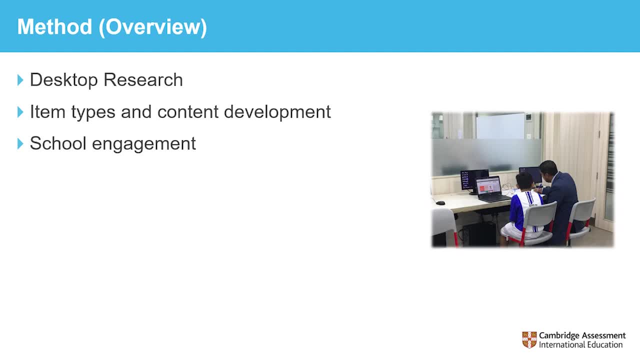 sourced from past assessment material. Thirdly, school engagement occurred. This was a vast piece of work covering our key markers, engaging schools to participate both remotely and in the face-to-face element of this work. Following this was a period of creating the on-screen assessment materials for the children. 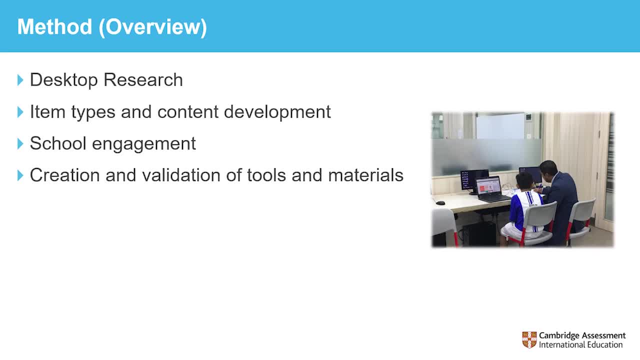 aged six to seven and eight to nine, with the associated tools and materials required for teachers to carry out the testing remotely and to feedback. There was a period of internal validation. After this iteration, one test materials were sent for remote testing. The group followed by a period of data analysis. 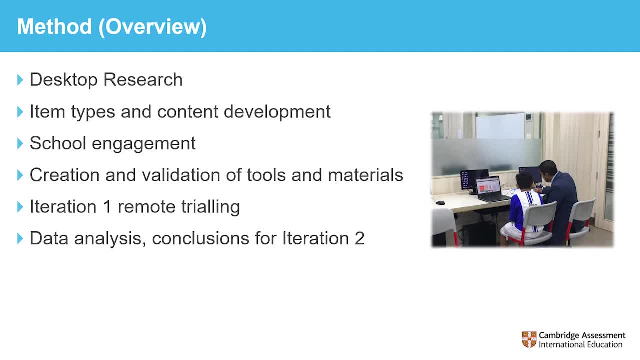 Data analysis occurred and conclusions for iteration two were made. From this we were able to create a second iteration of the on-screen assessment materials and the associated observation tools. These were trialled again, with improvements made both remotely and face-to-face. validation piece. 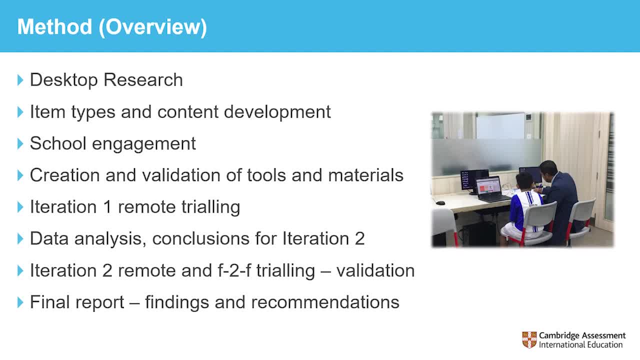 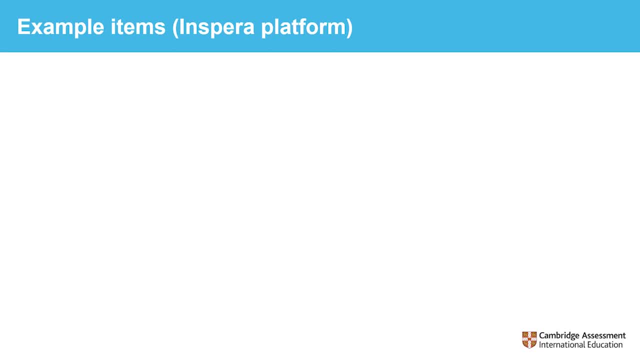 On receiving all data. the findings and recordings were received with this example. The results appeared to be: recommendations were made. as mentioned, we're using the inspira platform. here are some examples of the item types we used. firstly, gap match to order numbers. secondly, here's an example of a slider where you can position the arrow on the 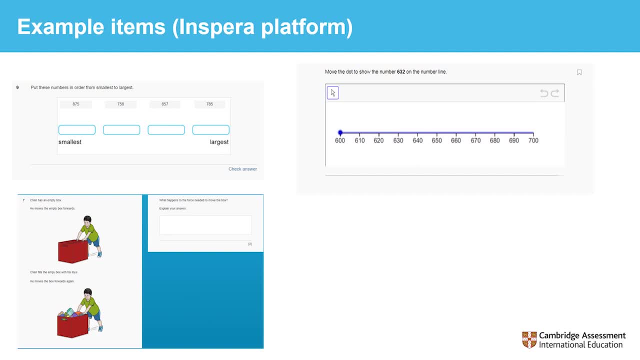 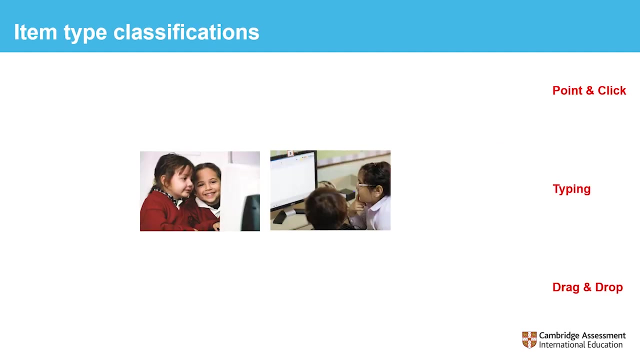 numbers. thirdly, an example of an extended text box where the learner is required to type. fourthly, a gap match onto an image, so pulling down tokens to actually sit on the image. item type classifications: as previously mentioned, all of the item types used in iteration. one of the on-screen assessments were 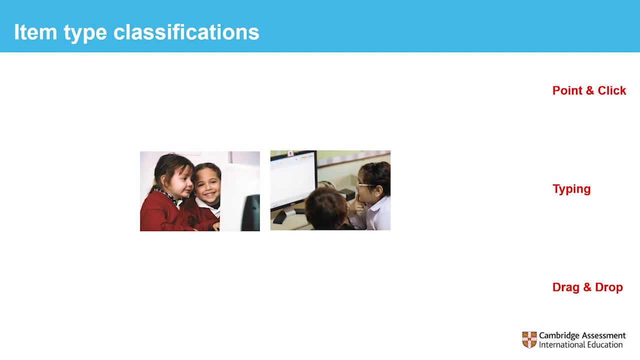 classified according to the actions that the learner would have to undertake: the item type. therefore, the item types used were classified as an item type. as we can see here we have the item type. that is as follows: Within the point and click category, we had both multiple choice. 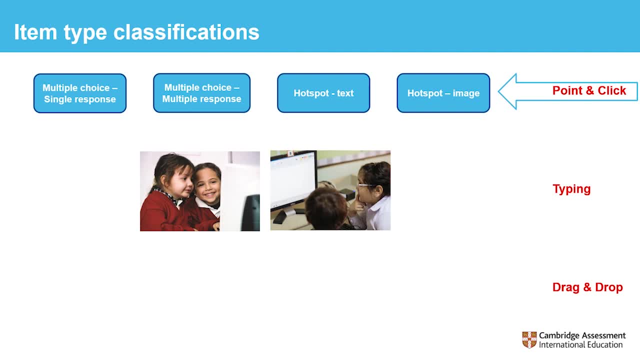 single response and multiple choice. multiple response items: hotspot on text and hotspot on an image. Within the drag-and-drop section, we had gap match onto an image, gap match onto a text using a slider and ordering. Finally, within typing, there were the extended text entry and text entry, which also 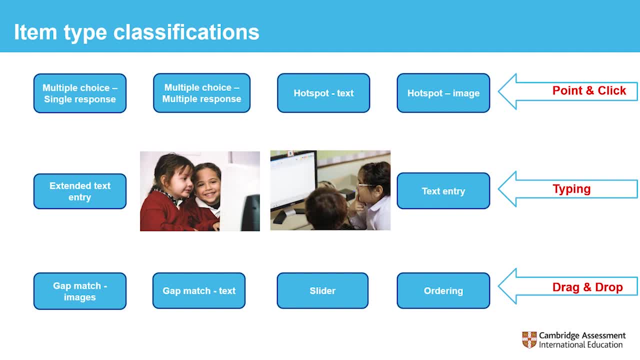 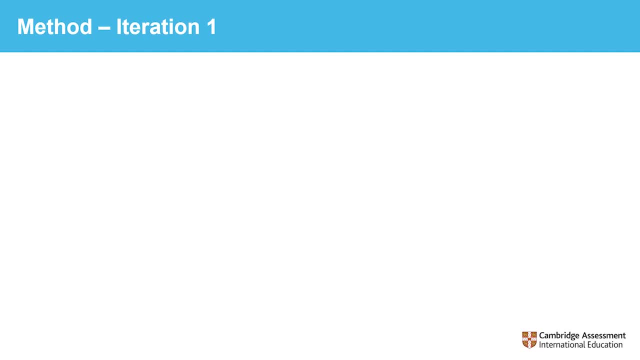 included short and numeric entry or entering small numbers. So the method for iteration 1.. The aim of this was to gain an initial understanding of how learners of the target age group interacted with certain item types and for us to understand if there are any that we could remove from. 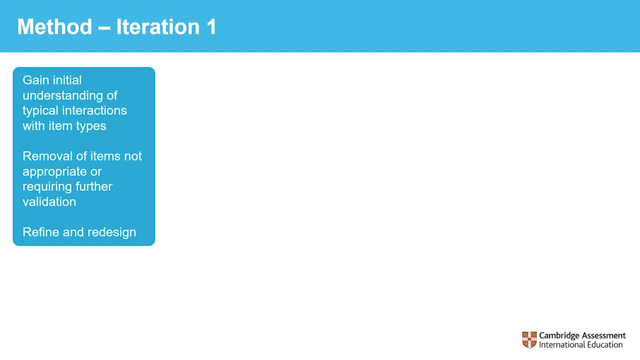 this early stage that were not suitable for younger learners, so that they could be removed or required further validation. It also allowed us to refine and redesign elements of the on-screen assessments we had created. During this phase, the on-screen assessment materials were created within INSPRA. 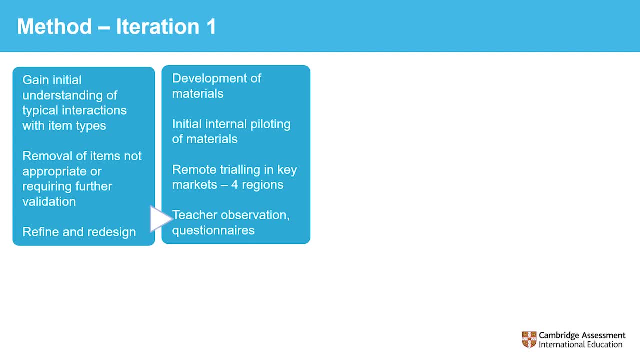 together with the associated observation schedules and associated instructions for teachers. As part of the QA process, these materials were piloted internally before the remote trialling occurred, across four regions On completion of the remote trialling, as well as teachers observing how their learners completed the items within the test. 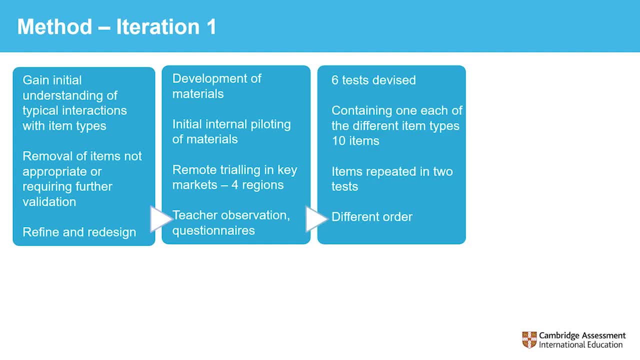 they were also asked to complete and send back questionnaires. In total, six different tests were devised and tested, each containing one each of the different item types and 10 items in completion. The order that the item types were presented were different within each of the six tests. 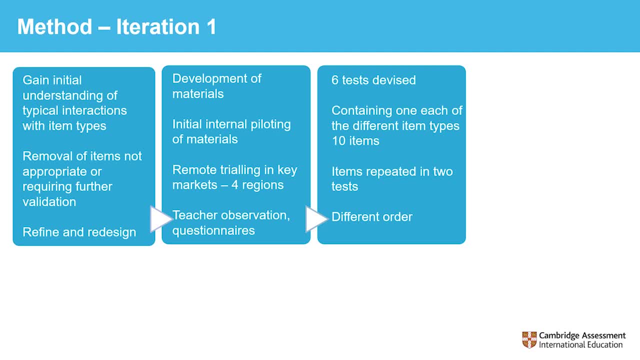 with a mix of maths, science and English content from practice. The results of the previous Cambridge tests were similar to the results of the previous Cambridge tests. The trialling occurred within eight countries across four regions. There were a total of 86 learners between the ages of six and nine, with 55 of them being male. 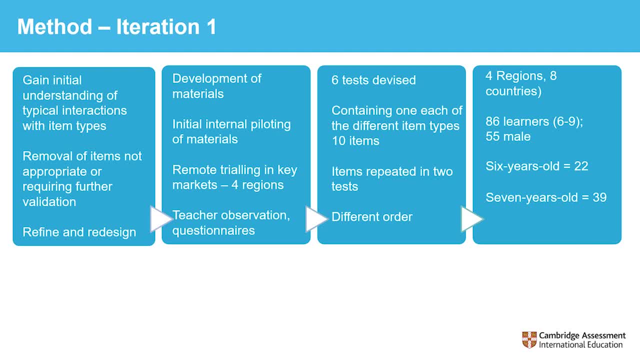 22 six-year-olds and 39 seven-year-olds. On completion, after analysis of the data and results gained from the first iteration, it was decided that the following items were needed: The results were to be removed as it was evident that learners struggled to interact with them. 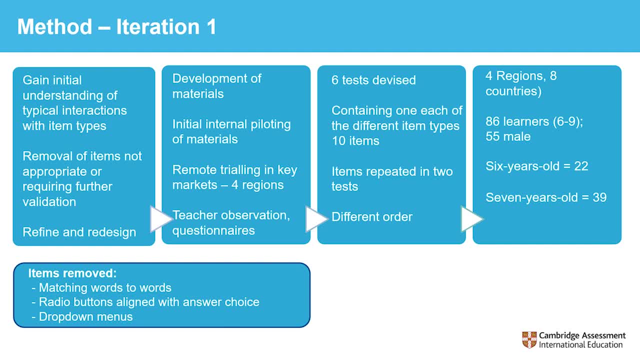 These were matching words to words, multiple choices of radio buttons aligned to the answer choice, and questions with drop-down menus. Changes that we made for the second iteration was that now there was only one test which contained 10 different item types. The content was also different from the first test, but still across the same three subjects. 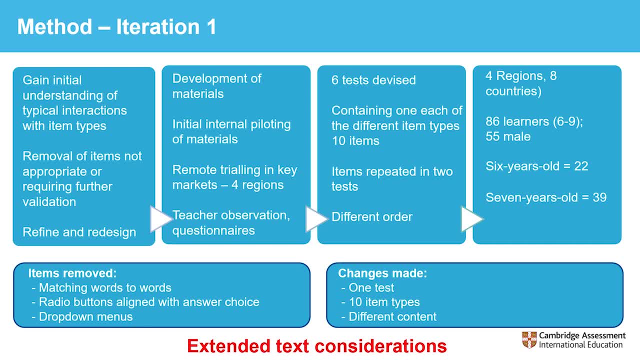 We did see from feedback and looking at item completion that the learners on the whole also had difficulty with extended text entry items, but these were kept in for the second iteration so as to gain a better understanding of what some of the issues were experienced with typing. 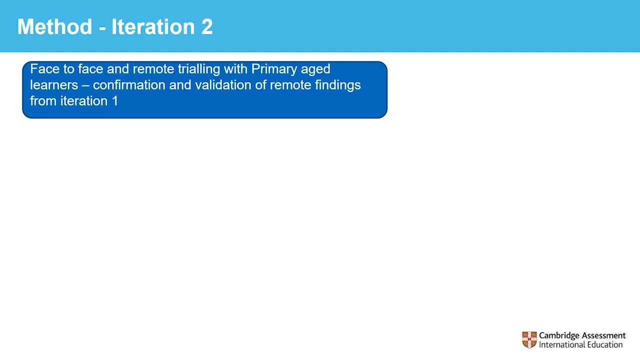 Method: Iteration 2. This incorporated the changes, as mentioned, from the outcomes of Iteration 1.. There were two forms of trialling again, the remote trialling, but also face-to-face trialling, with the aim of this being able to confirm and validate the findings from item type interaction from the first iteration. 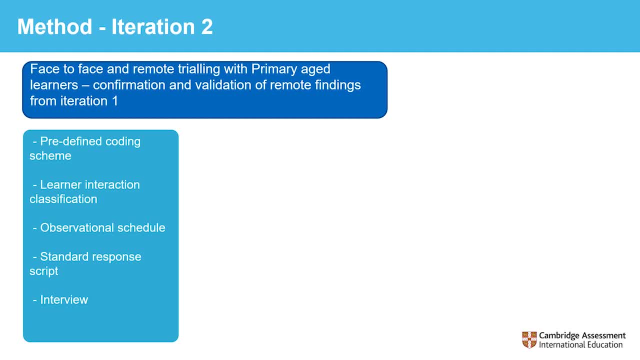 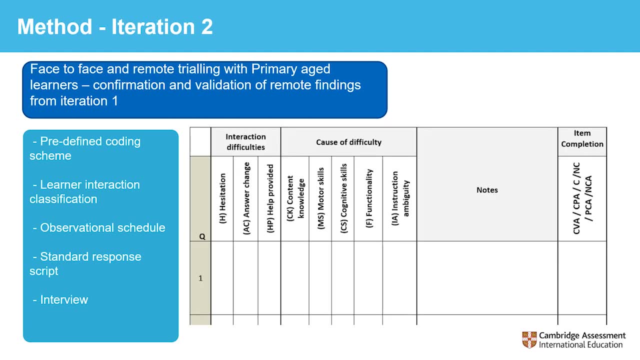 To support the face-to-face element of the trialling, an observation schedule was developed with research colleagues to use whilst observing learners doing the on-screen tests. as shown, There was a predefined coding scheme on how the learner attempted the item and space to record the perceived difficulty and cause. 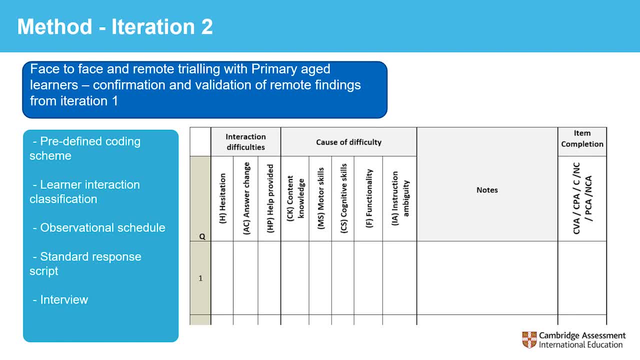 This coding system was standardised between colleagues who were observing and rehearsed Learners' interactions were classified as either completed. completed with verbal assistance, completed with physical assistance, partly completed with assistance, not completed with assistance or not completed. Alongside this, to ensure consistency when interacting with learners, 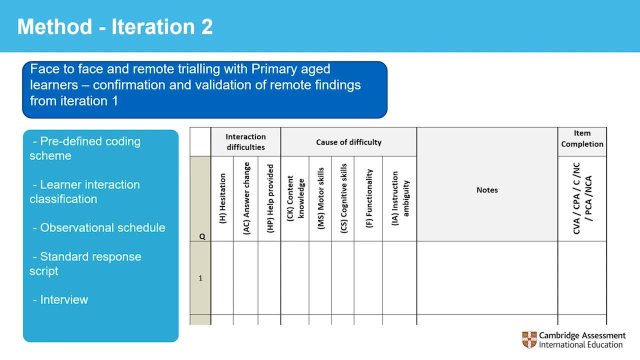 a standard response script was created so that colleagues who were testing were responding in the same way to the learners' questions. Following testing, the learners were interviewed on aspects of the test and also their use and understanding of digital inside and outside of the classroom. 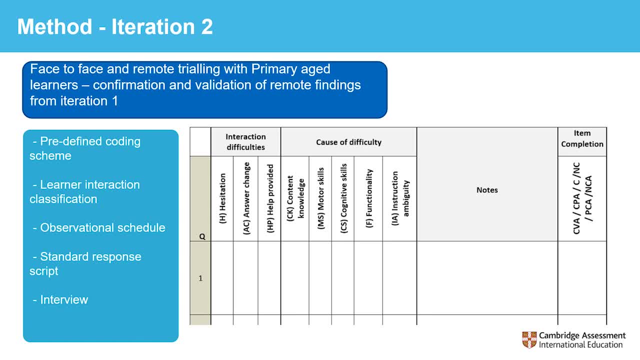 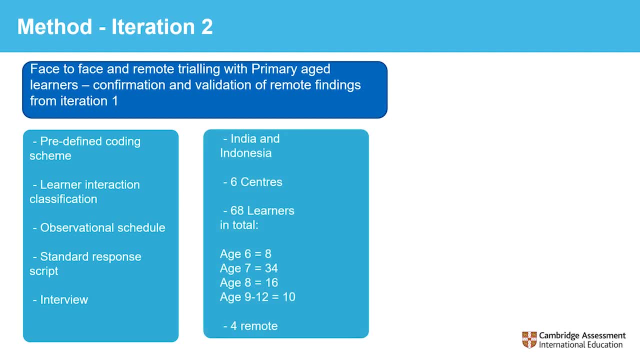 There was also remote trialling occurring at a school in the UAE with four learners. For the face-to-face trialling schools in Mumbai, India, and Jakarta, Indonesia, were used In total six centres, three in each location, 68 learners of the shown numbers in each age group. 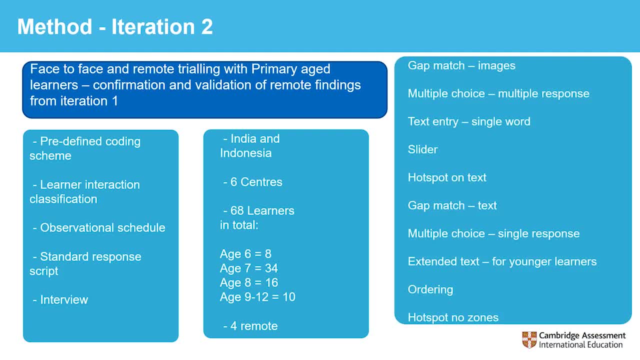 The item types tested within the test were: gap match images, multiple choice multiple response text, entry with single words, slider, hotspot on text. gap match text- multiple choice- single response, extended text for younger learners, ordering and hotspot with no zones. 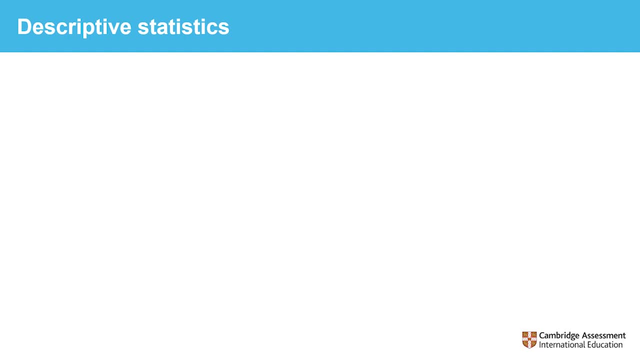 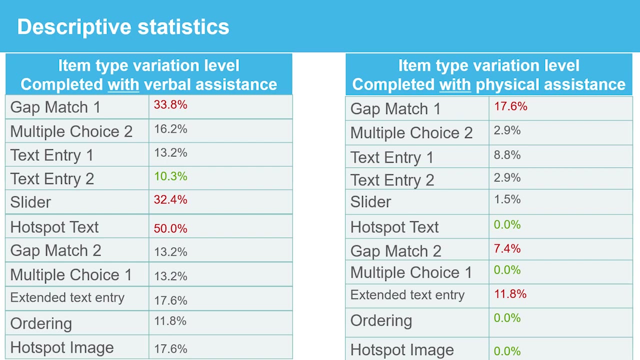 My colleague carried out statistics on the results and summarised as follows. The descriptive statistics showed that: verbal assistance- according to the data- all of the items. for all items. a certain percentage of learners were only able to use verbal assistance. verbal assistance according to the data- all of the items. for all items. a certain percentage of learners were only able to use verbal assistance. 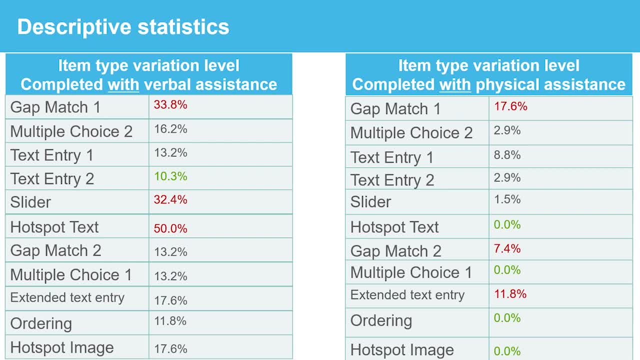 way, they were only able to complete with adult verbal assistance. In other words, unlike the selection of items for which no learner required physical assistance, when it came to verbal assistance, at least 10.3 percent of learners required some form of help from an adult across the board. 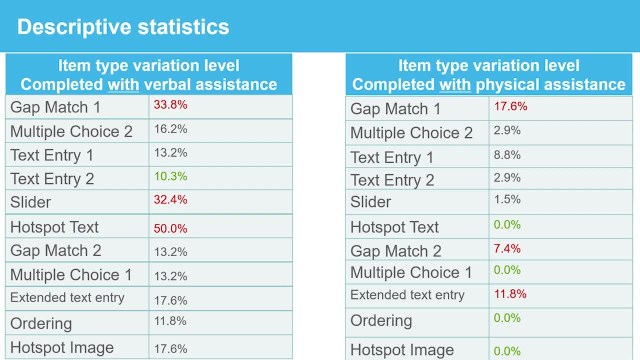 Hotspot texts required the most verbal assistance. qualitative data highlighted that this was due to learners not understanding how to choose the word in order to answer the question. This suggests that the command word and presentation of the item types was unclear, as learners did not know which action was expected of them. to choose Some. 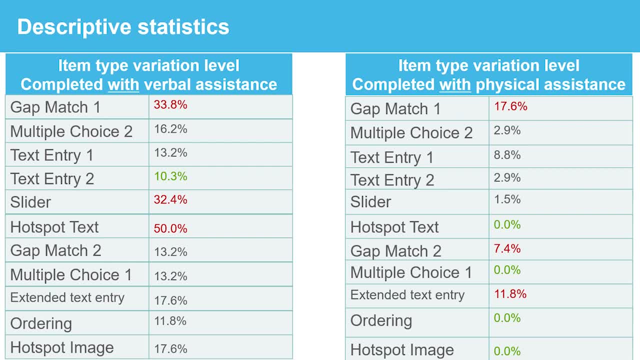 learners tried to highlight the word, which should be considered for future designs of this item. type Match 1 may have slightly inflated rate of learners requiring verbal assistance as this was the first question in the test. Qualitatively, this is supported by the observation notes as learners generally 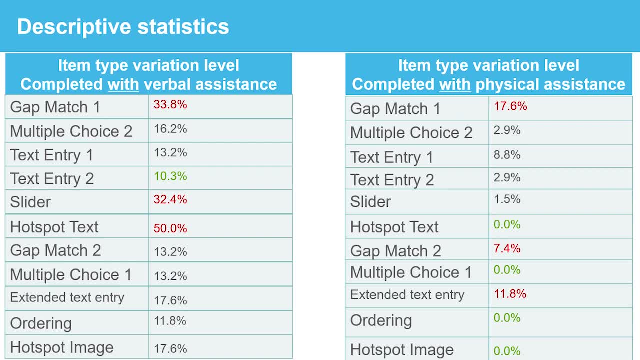 asked the adult a question which suggested they knew what was expected but was seeking reassurance. The cognitive loader slider may explain the higher percentage of learners who required adult guidance for this item type. Another explanation that these findings may relate to language: Completion of this question without assistance was rely on the learner understanding the 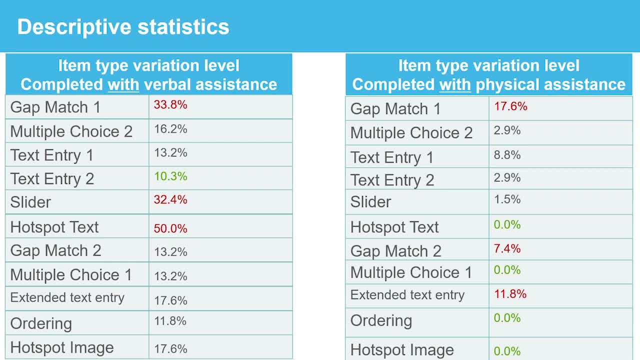 word dot in order to know what to move. Physical assistance: Learners did not require physical assistance completing hotspot text, multiple choice one ordering or hotspot image. This suggests that, the exception of multiple choice one, young learners have the necessary motor skills required to. 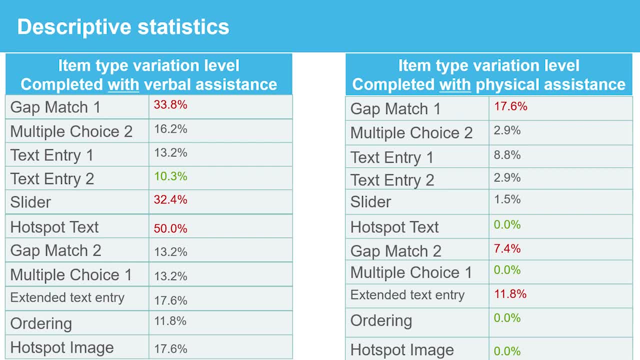 complete point-and-click items without assistance. Ordering may reflect learners familiarity with the drag-and-drop interaction. as this was the penultimate item in the test For the other drag-and-drop items, some learners required physical assistance, with 17.6% of learners completing their 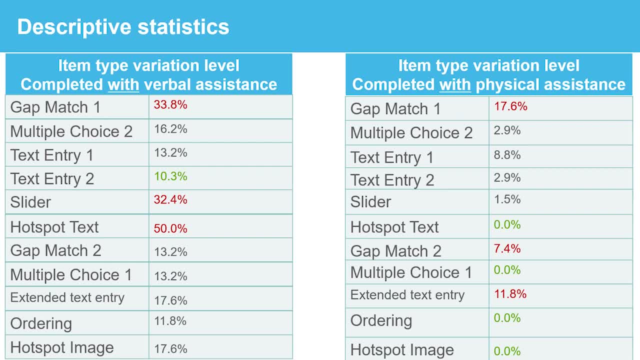 interaction with an adult, inputting their answer. for them for match one and 7.4% for match two. Learners did not require physical assistance. completing hotspot text. multiple choice one. ordering hotspot image. This suggests that, with the exception of multiple choice one, young learners had the 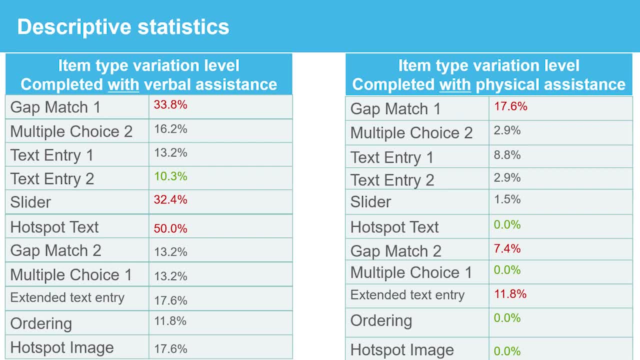 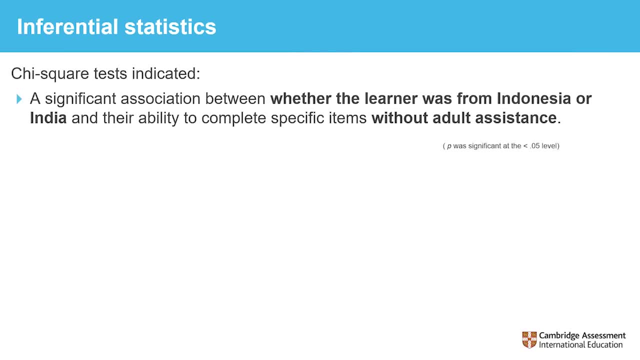 necessary motor skills required to complete point-and-click item types without assistance. Inferential statistics. Using inferential statistics, it showed that a chi-square test indicated that there was a significant association between whether the learner was from Indonesia or India and their ability to complete specific. 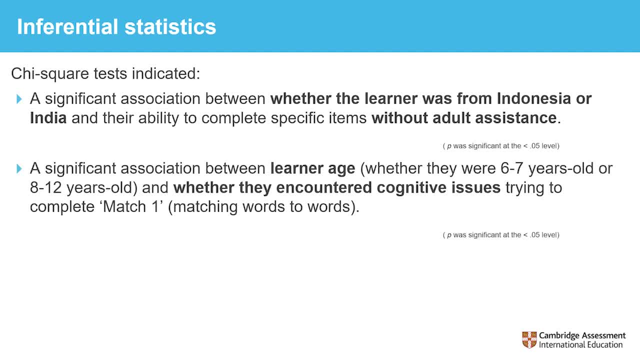 items without adult assistance. it was established that there was a significant association between learner age, whether they were six to seven year olds or eight to twelve year olds, and whether they encountered cognitive issues. trying to complete match one matching words to words, a three-way log linear analysis was also done, looking at the item type against adult. 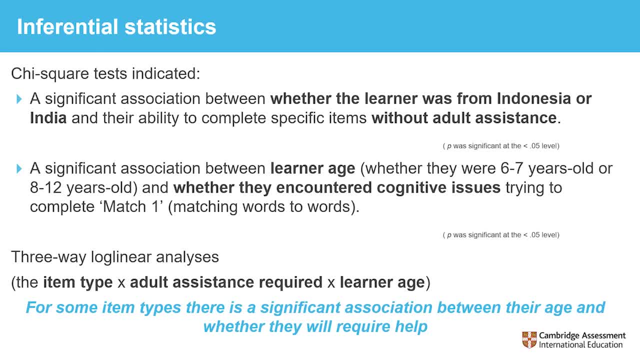 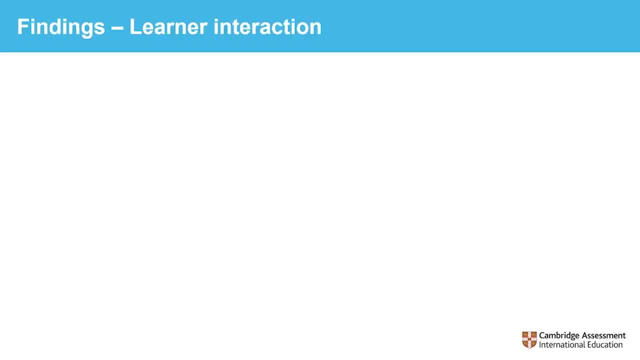 assistance required against the learner age and it was concluded that for some item types only there was a significant association between their age and whether they would require help. so next i'll talk about what we found out in terms of the learner interaction. it can be concluded that overall, the younger the learner, the less developed their cognitive. 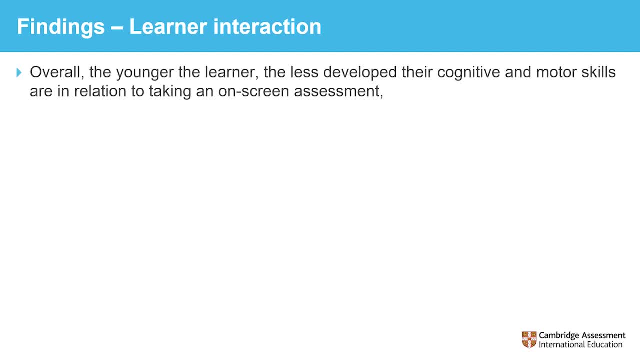 and motor skills are in relation to taking on-screen assessment and interacting successfully with all items that were presented within the platform. it was evident that there was a gradual decrease in the amount of adult assistance required to complete match one matching words, and it was also concluded that, for some item types, 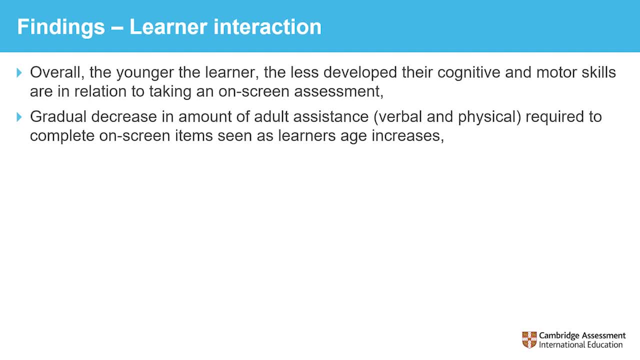 there was a gradual decrease in the amount of adult assistance required, both verbal and physical, to complete on-screen items. seen as learners age increases or the older the learner is, there was a significant association between the learner and whether they required assistance with different on-screen item types, for example, younger learners finding point-and-click items. 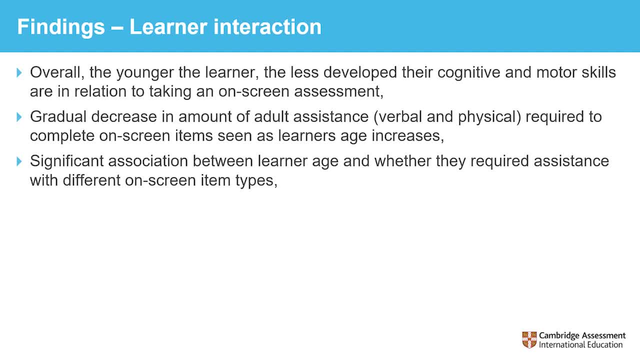 more easy to interact with compared to typing an extended response. learners required adult assistance with certain on-screen item types more so than others, for example, the hot spot on text. younger learners aged six to eight required most assistance with drag and drop and typing. there are significant regional variation in learners abilities to interact with on-screen. 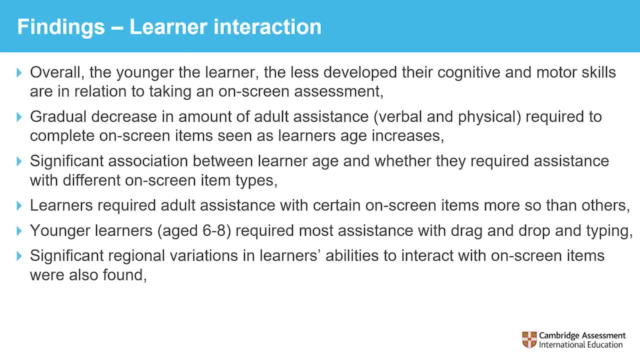 items. this was more prevalent when looking at the data from the face-to-face trialing specifically, learners from india required more verbal and physical assistance than learners from indonesia, suggesting this is due to the differences in learner context and experience, for example, their exposure to one screen and experience practicing digital literacy skills typing. 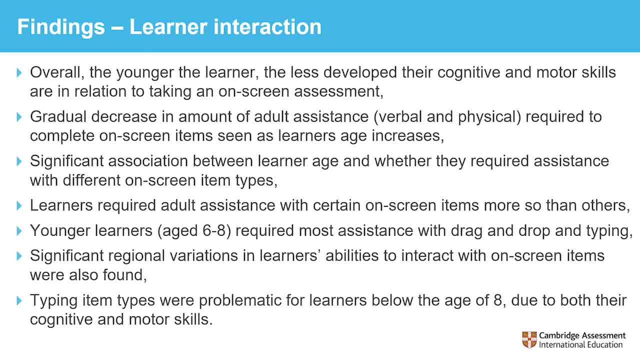 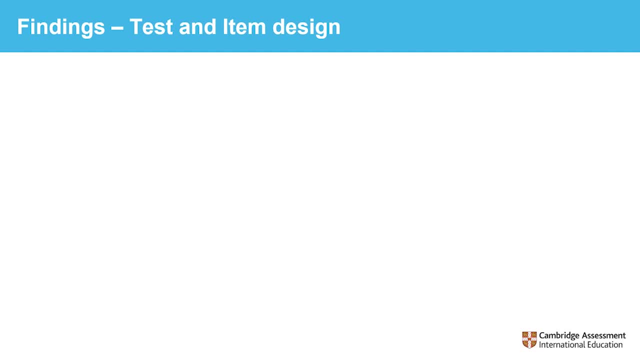 items were problematic for learners below the age of eight, and this was due to both their cognitive and motor skills potentially not being as fully developed as required. a lot of young learners were seen to hunt and peck for letters on the keyboard with one finger. there are also findings and conclusions that can be. 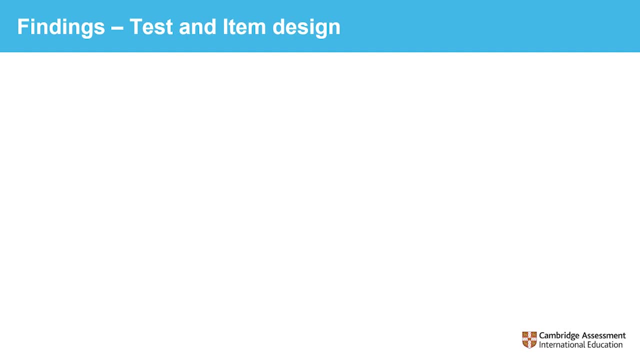 drawn with regard to the design and the test and items within it. the overall on-screen assessment design relates to the content and location of items and order they appear in may affect the learner's ability to successfully complete certain items. therefore, going forward, should there be, should there be, consideration of where these are? 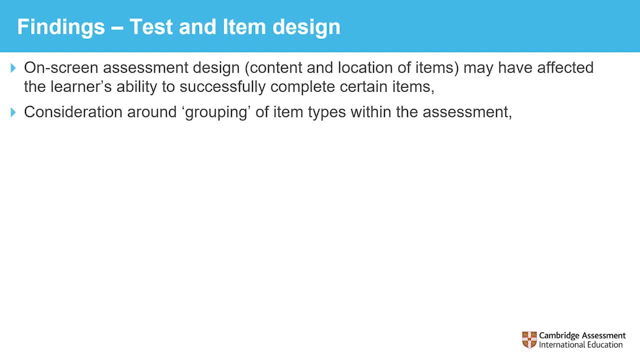 consideration around grouping of items within the assessment, such as all the other ones and the point and click category first, followed by drag and drop items, followed by typing. would this work better? fairness is a key consideration when designing any on-screen assessment for young learners, to ensure your learners with cognitive and motor skills that are less developed are not 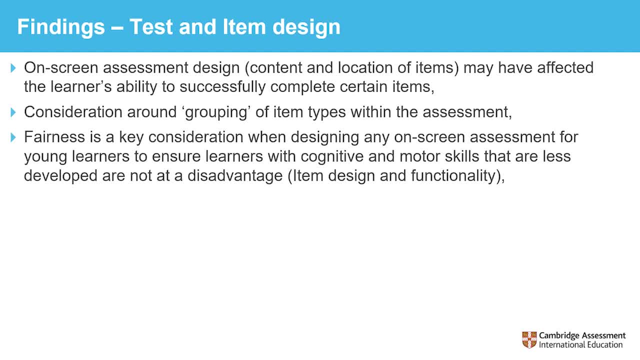 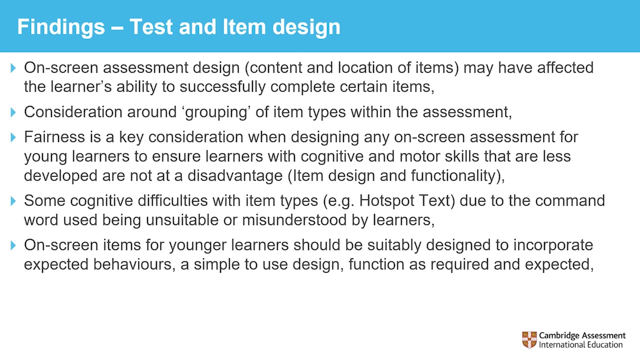 disadvantaged. again relating to the. this relates to the item time type, design and functionality. it can be summarized that some of the cognitive difficulties with item types, for example hotspot text, were due to the command words used being unsuitable or misunderstood by learners. do these need to be more specific? on-screen items for younger learners should be suitably. 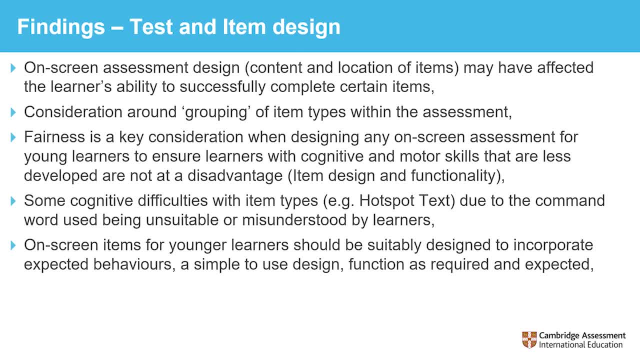 designed to incorporate expected behaviors. a simple to use design function, as required and expected, based on a child's prior knowledge and experience of items similar in other contexts, whether this be in the teaching learning space or other digital products being used, is essential for learners to be familiarized with assessment materials by using some 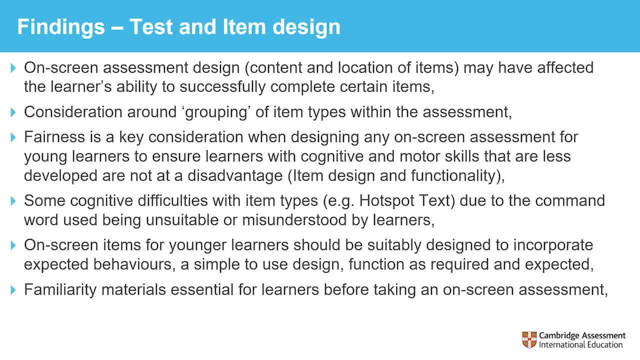 type of familiarity material before taking an on-screen assessment that will show them the item type, functionality of items that they're going to be exposed to and any on-screen design and tools, together with the overall user journey that they will take. through the test, certain items can be dismissed as being suitable for young learners. 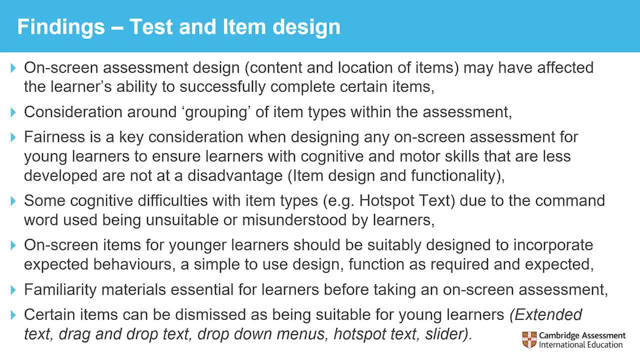 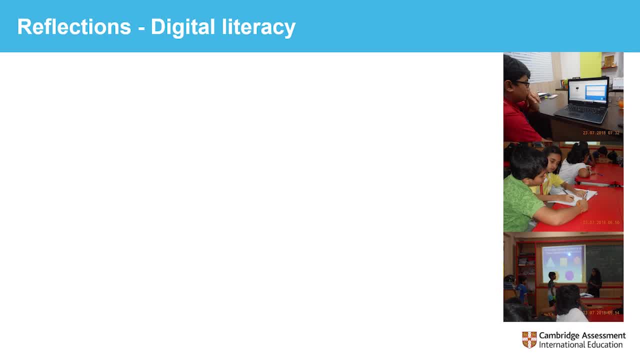 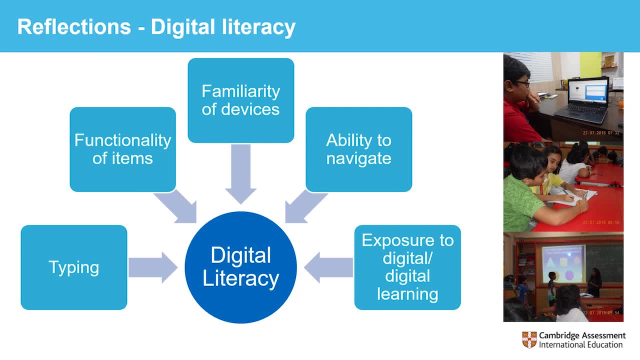 as well as for those who are not yet familiar with the concept of digital literacy. we can look at some examples, such as the extended text, drag and drop with a text, drop-down menus, hotspot text and slider. on reflection, one area that stood out was digital literacy amongst learners. 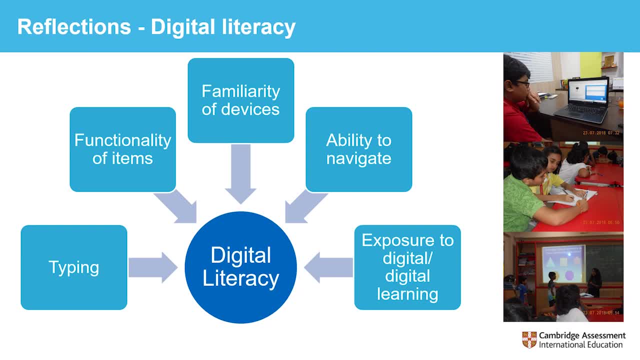 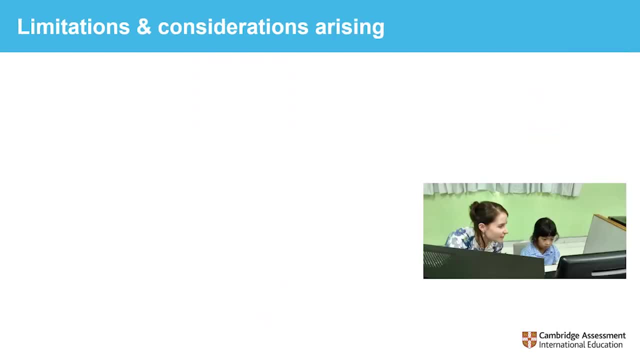 we can't assume that a seven-year-old in one country has the same ability in terms of digital literacy as another. this was quite evident between learners observed during the face-to-face trialing in indian schools versus those in indonesian schools. some of the limitations and considerations that arose: 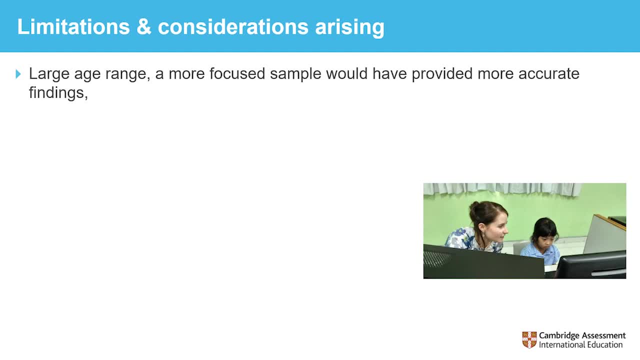 included the. the sample overall had a large age range. a more focused sample would have provided more accurate findings. the cognitive issues have not been assessed psychometrically, but inferred through the help. learners asked for whilst taking the test and their observed challenges learning potentially were not familiar with the device and the on-screen assessment platform.